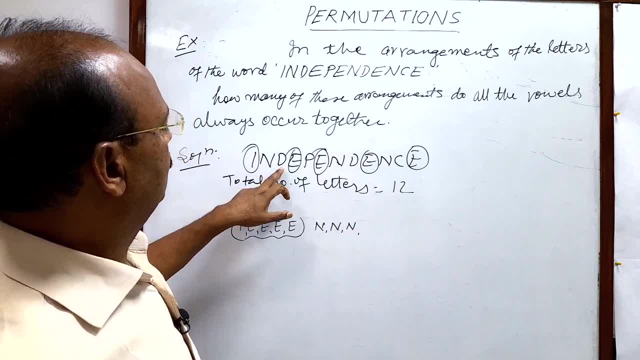 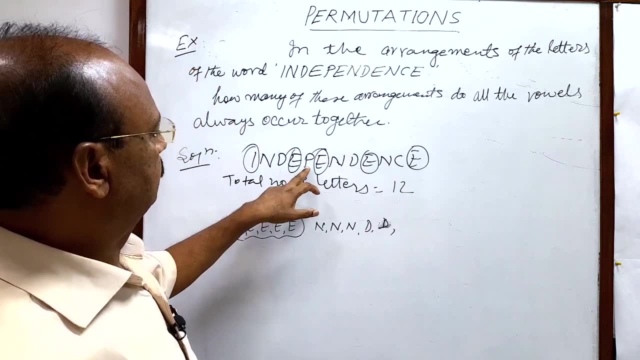 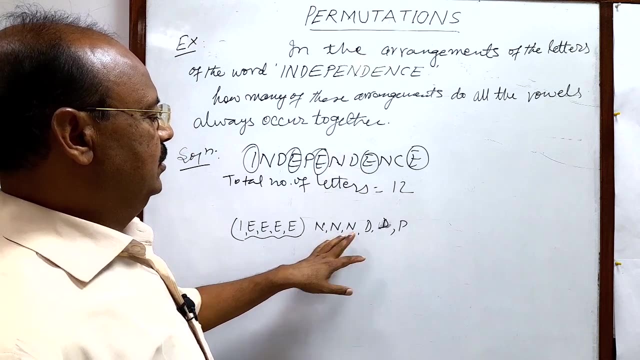 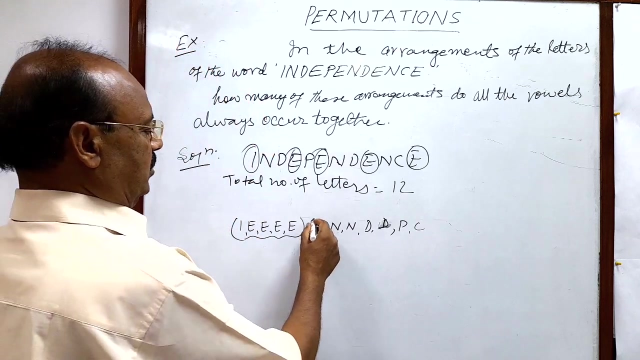 And two D. One D is here, One D is here. We have two D And P is one. Total five, Five and three, eight, nine, ten, eleven, and one letter is C. Okay, So this is group of N, This is group of D. 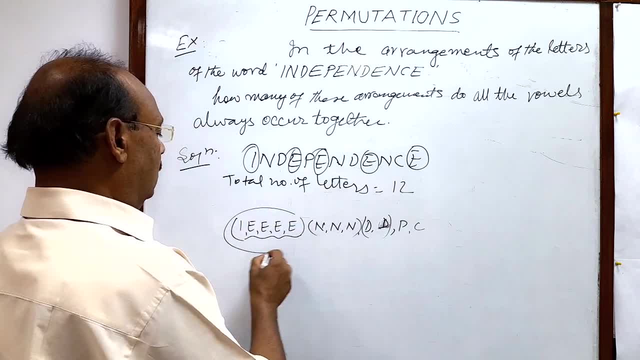 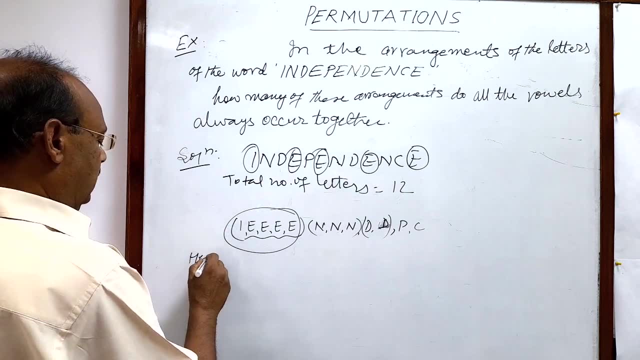 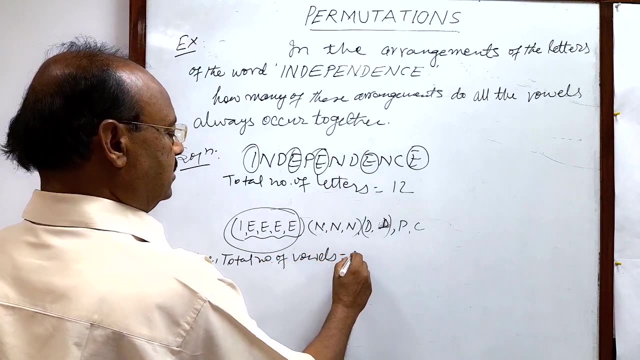 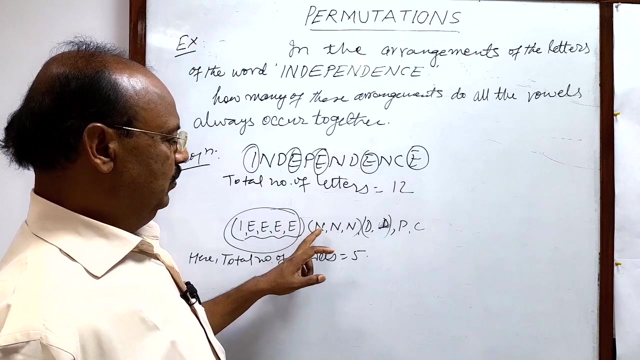 Arrangements can be made when we have to keep all these five vowels together. Okay, So here we see that here, total number of vowels, Total number of vowels is five And this will be treated as one group. So we are having one plus this three. One plus three is four And two. 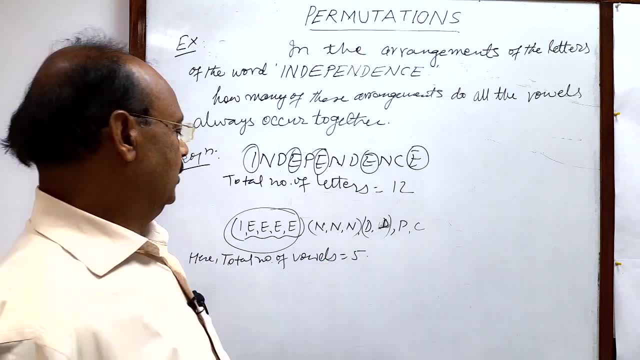 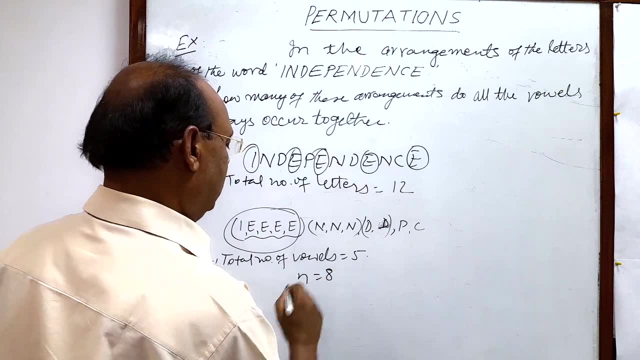 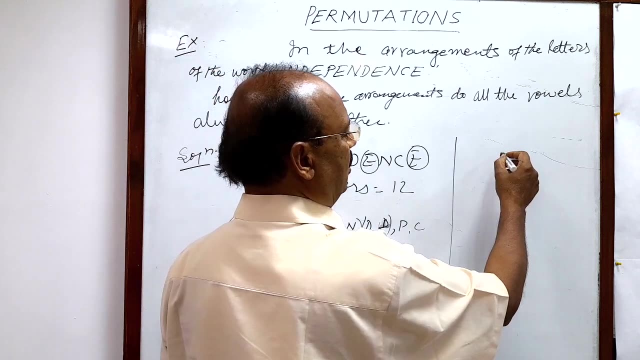 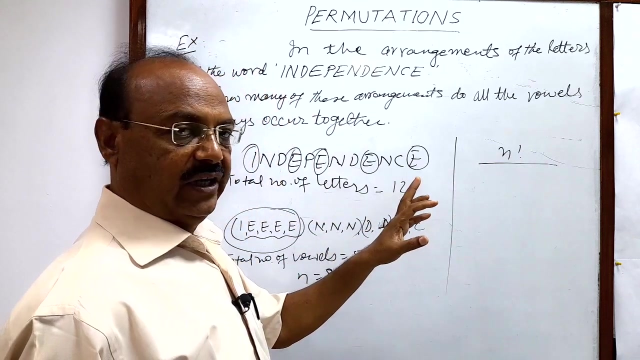 Six and two Eight. Okay, So N is equal to how much? here N is equal to eight. Okay, N is equal to here, eight. And we know the formula- We have discussed it several times in another videos also- That here we will use the formula. Number of arrangements will be N factorial. This is two factorial of total number of objects. But here we have to take care that this will be counted as one, Because this is a single group. 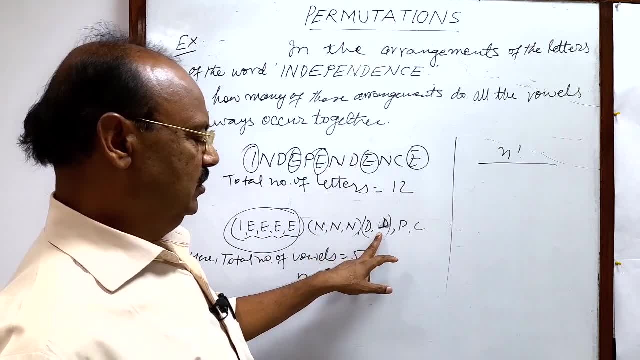 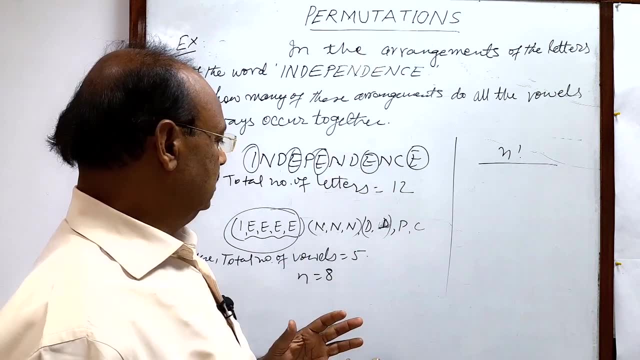 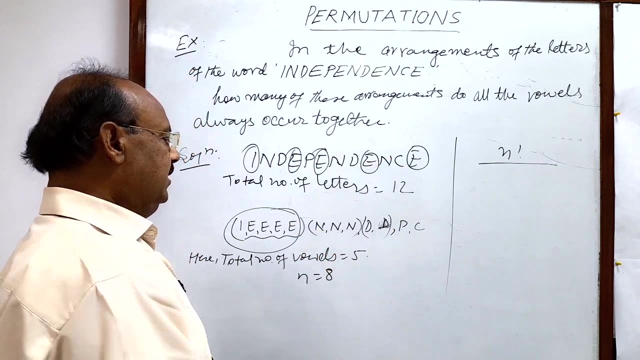 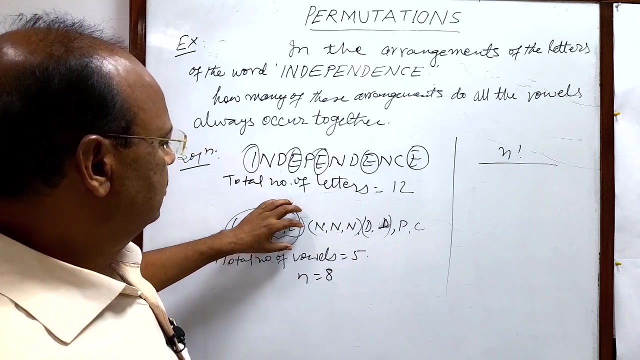 So one and three, four and two, Six, seven, eight. So N is equal to eight And there are some like letters, As for example, three Here, two, Okay, So this will be divided by this factorials of like letters, But this will be as a single letter. So we will not divide this N factorial. 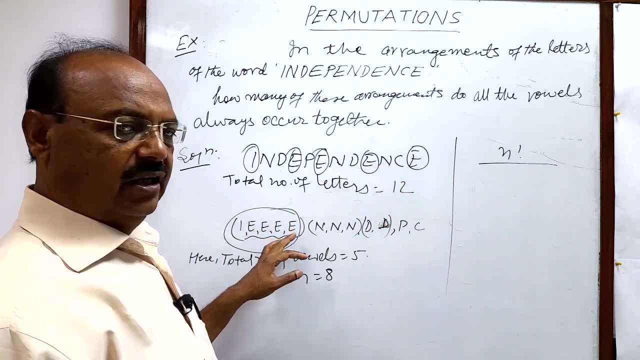 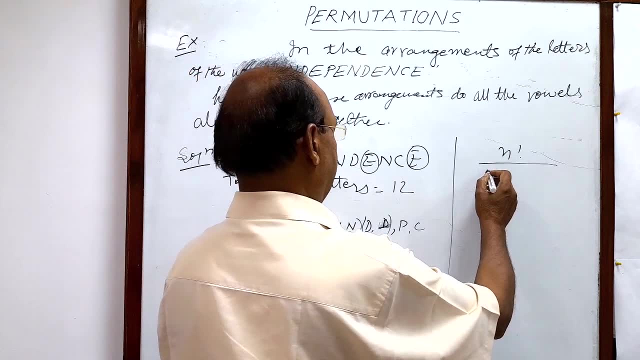 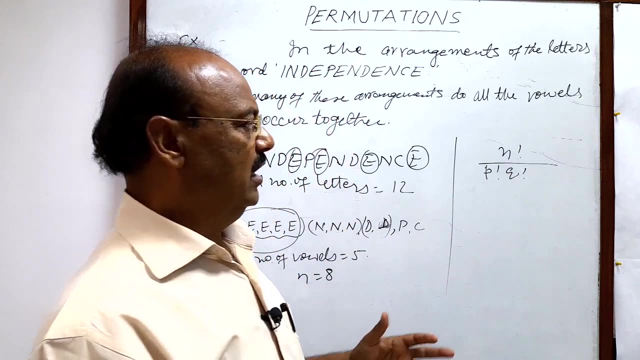 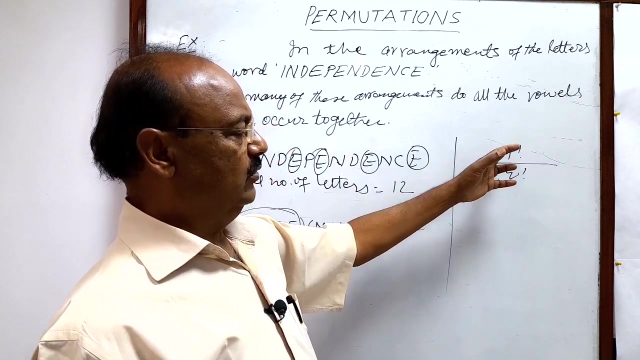 By four factorial, Though four is are here Because we are taking this group as a single object. Okay, So three N's are here, So divided by three factorial. Here, as a formula we will write P factorial, Q factorial, like this: Where P letters are alike, or P objects are alike, Q objects are alike, So if number of alike is here, then N factorial will be divided by factorial of the alike objects. Okay, So in this case, 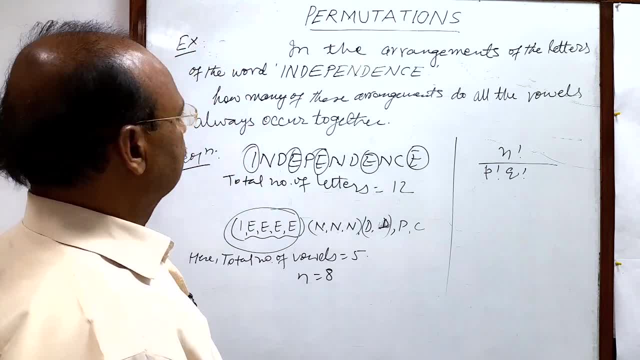 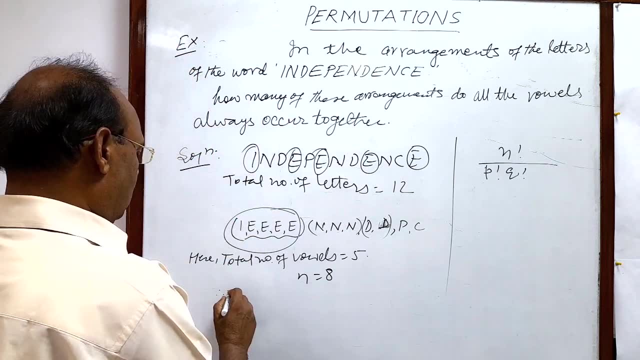 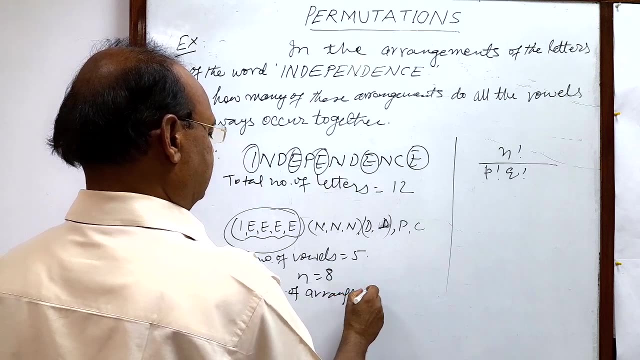 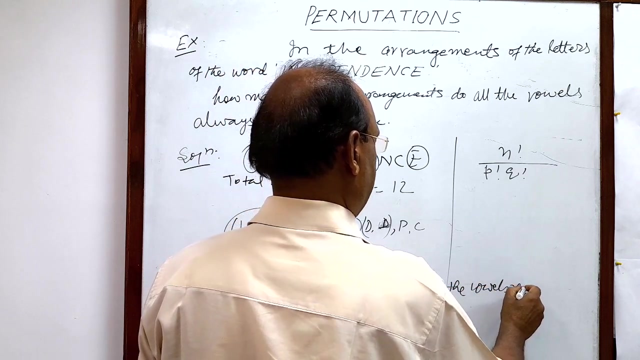 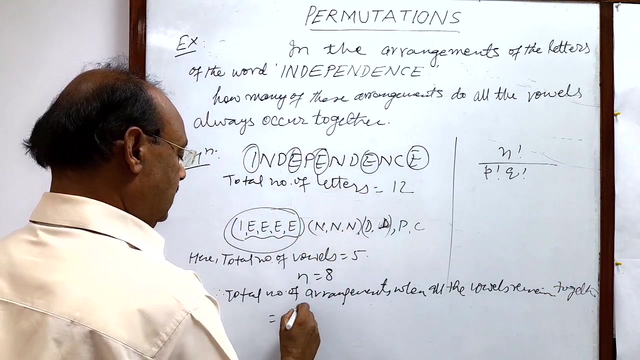 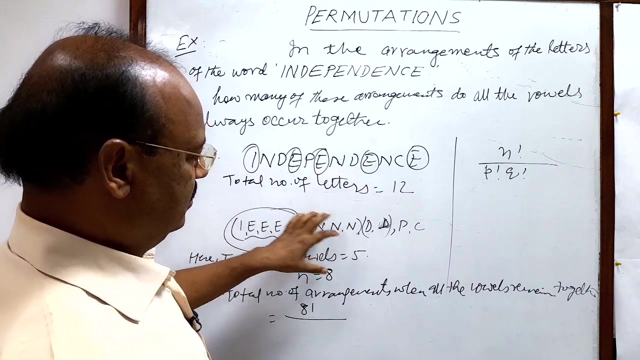 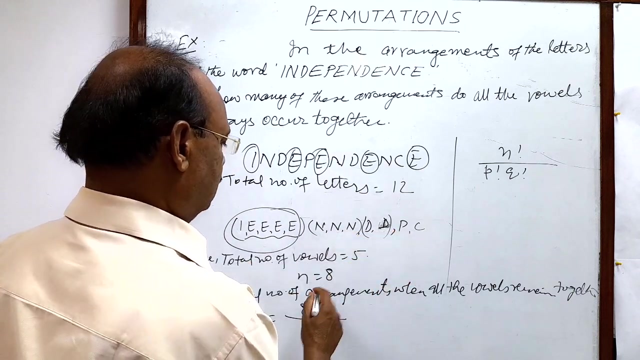 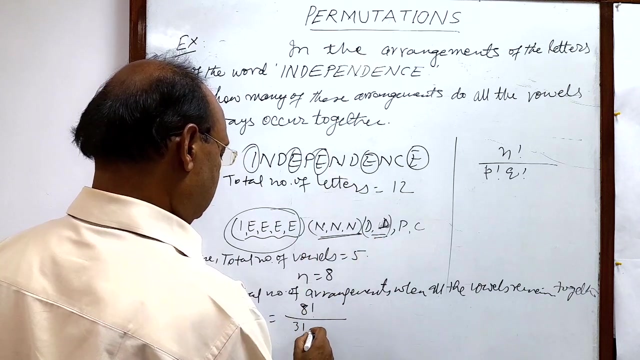 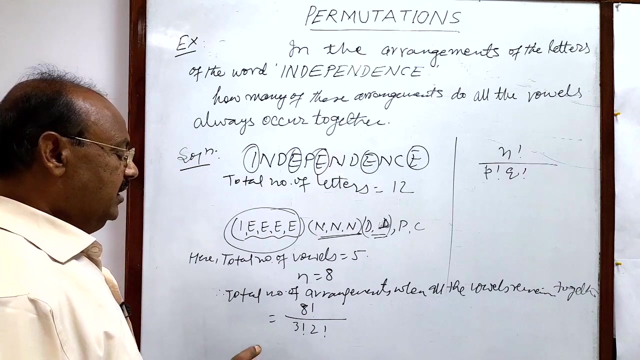 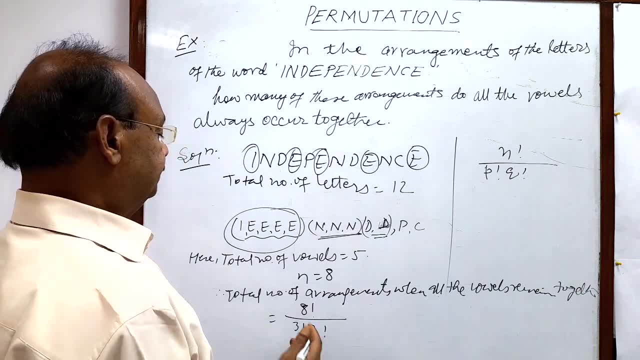 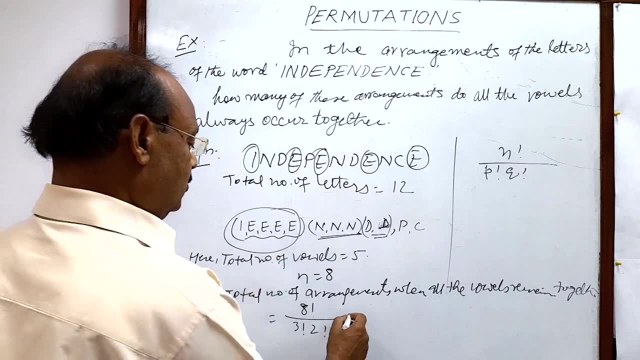 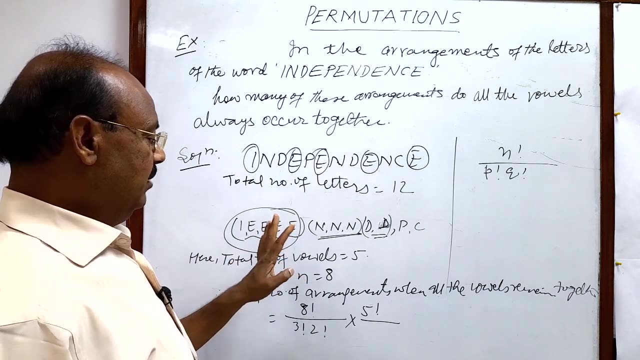 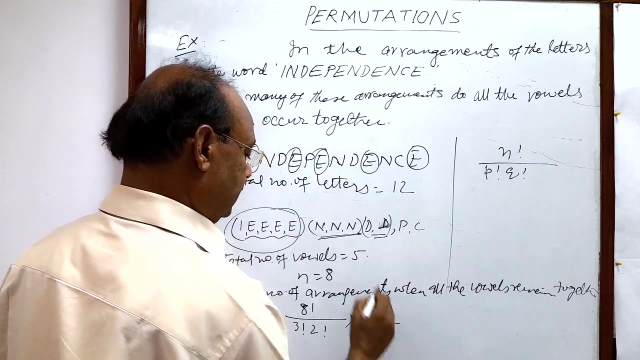 chances, chances here, that all the balls remain together. but there is also a scope of elements. five letters are here, so this will be multiplied with five factorial and out of this five letters, we have same elements. e how many times four times four is, are here, so divided by four, factorial hope. 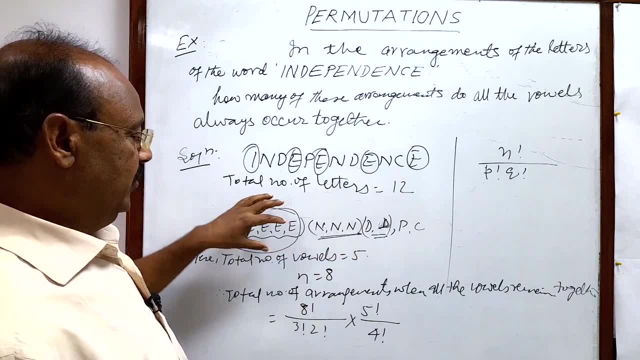 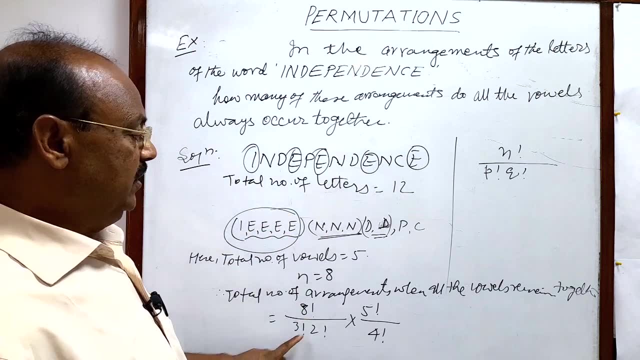 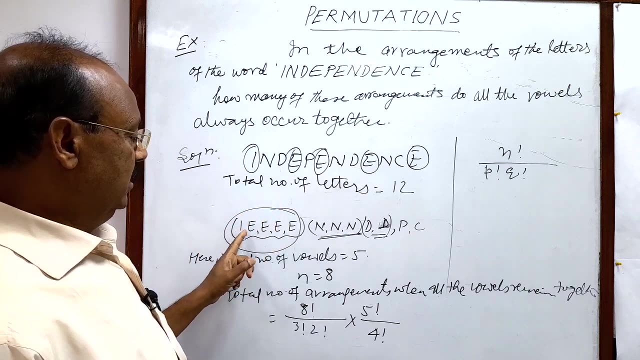 you have understood, is 80 total number of objects when this group, num, group of vowels, is taken as a single object. so this is 8 factorial 3. n is here, so divided by 3 factorial 2. D is here, so divided by 2 factorial. again, there is a scope of arrangement in this group also. so total number: 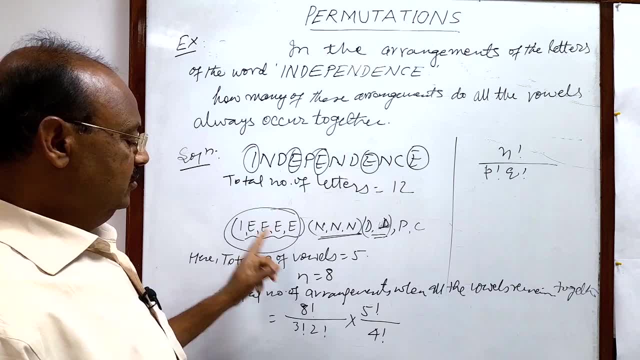 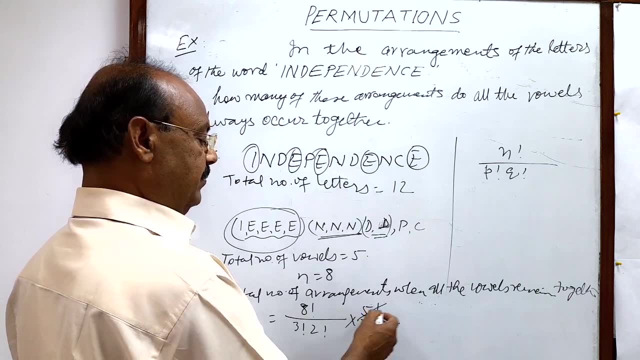 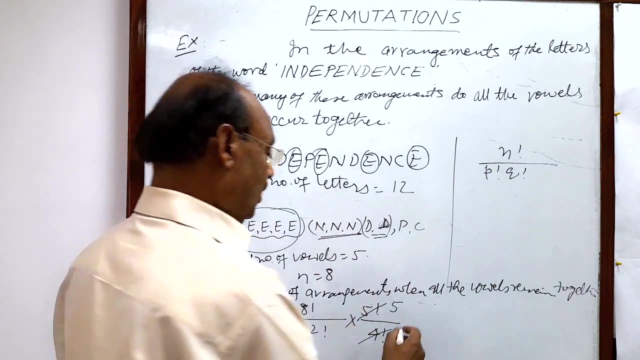 of objects is 5, so 5 factorial and there are 4 e, so divided by 4 factorial. ok, so after calculation we will get the result: this 4 factorial we cancel out with this 5 factorial. 5 will remain here because 5 factorial can be written as 4 factorial into 5. 4 factorial we cancel out, and here this 8. 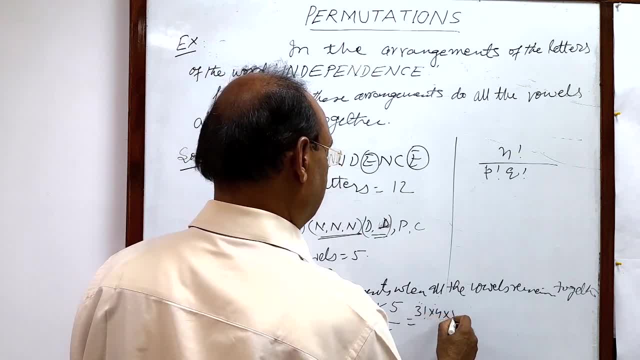 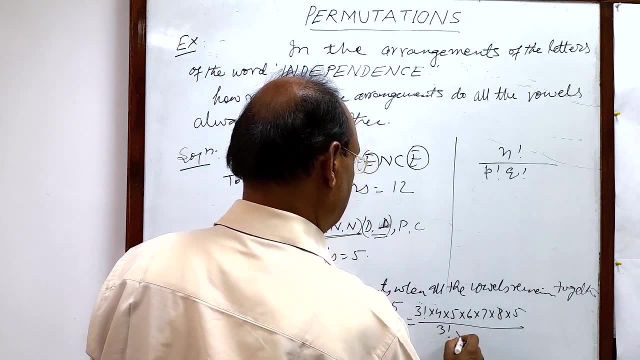 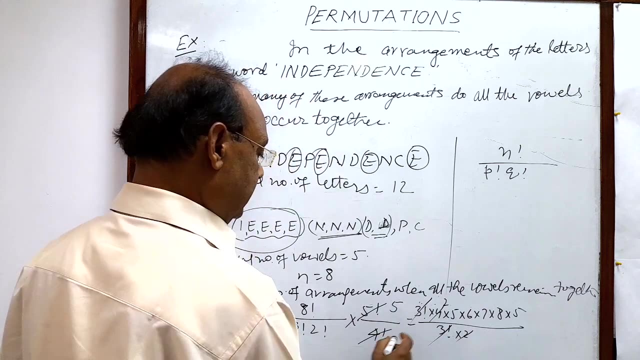 factorial can be written as 3 factorial into 4, 5, 6, 7, 8 into this. 5 divided by 3 factorial into 2, 2 factorial is 2. ok, so you cancel 2 to the 4. now let us multiply these numbers. numbers are 2 into 5.